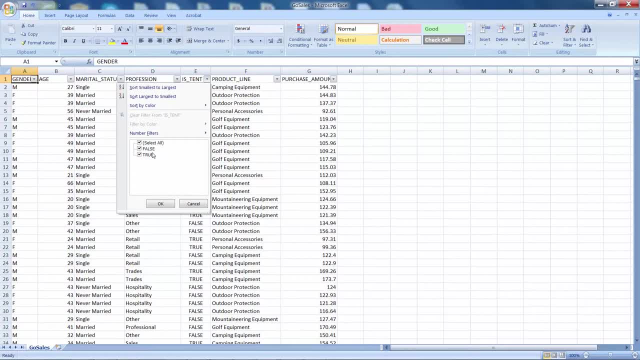 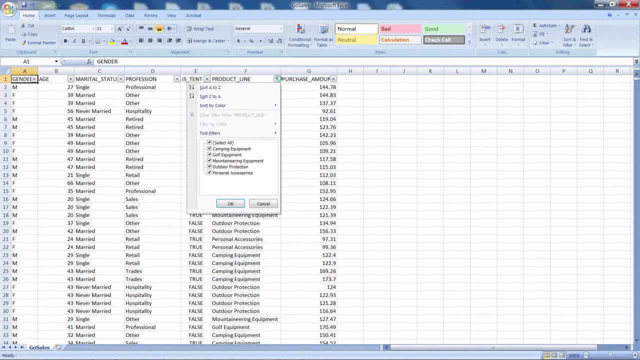 true and zero is false. So the answer to the question lies within these two boundaries. Now, if you want to train the model to make a prediction on a more complicated column such as the product line, so if I actually open the filter on the product line, it has many unique values. So you have 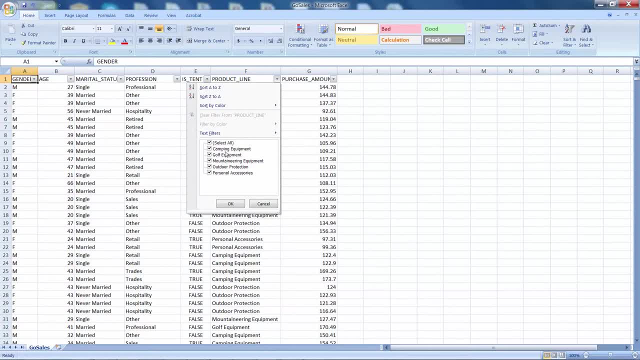 camping golf, mountaineering, outdoor personal. So that makes it five. So now you have to train the algorithm to pick one of these categories for a given profile. So, for example, female 49, married other. what is this profile most interested in? All right, now let's go ahead. 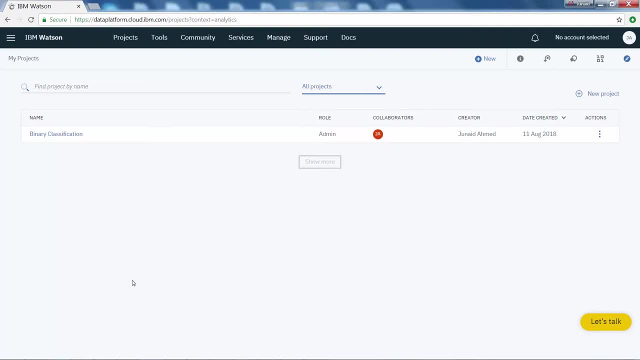 and build this. So I'm here on the Projects page Of my IBM Watson account. So if you have not logged in already, or if you want to, please log in, So I'm going to use the same project which I have used before, So go into the project. 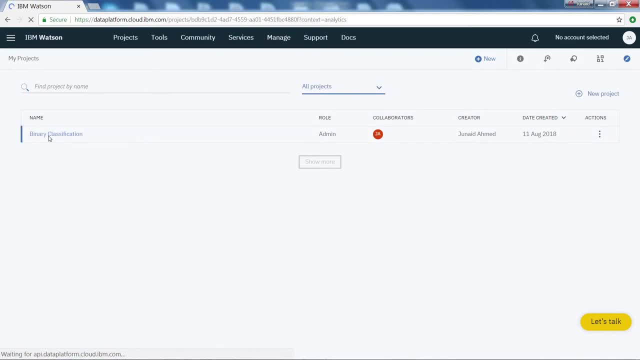 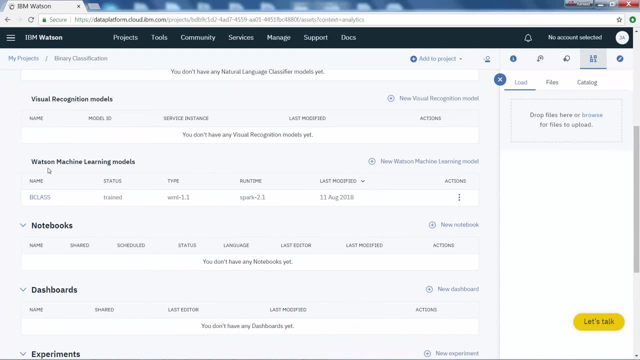 For me it is binary classification, And here I'm going to add another machine learning model. So go down here and find the Watson machine learning models. You can find your old B2B class model here, so click on what's in machine learning model here. give it a name. i'm going to 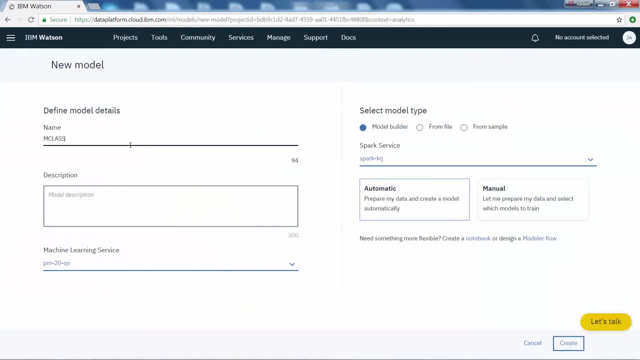 call it m class here and, as you can see, there is a machine learning service associated. there's a spark service associated. we're going to leave it at the model builder and this time we're going to change it to manual. so this allows you to choose the algorithm you want to use. so let's say 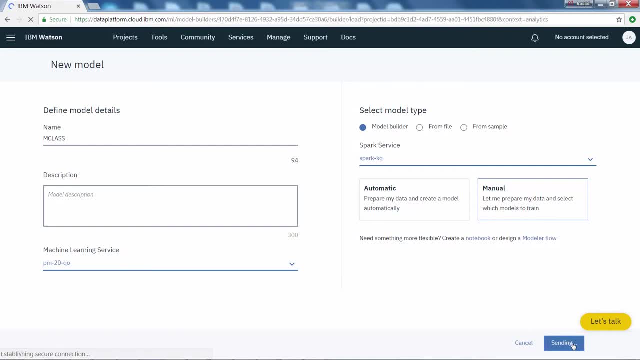 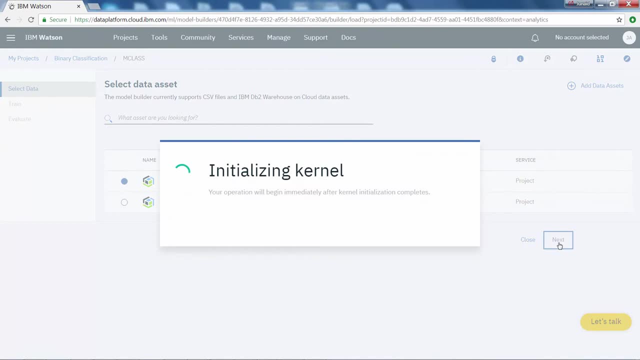 create. you're going to be using the same go sales data, so select go sales jet and say next: now of course you can use other data. if you have a nice clean data set setting, then of course you can use that as well. so make sure you do some due diligence. 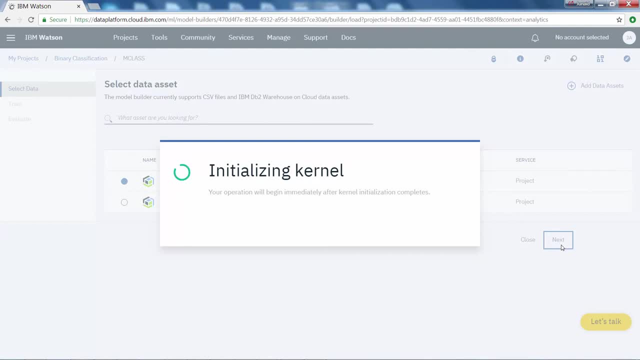 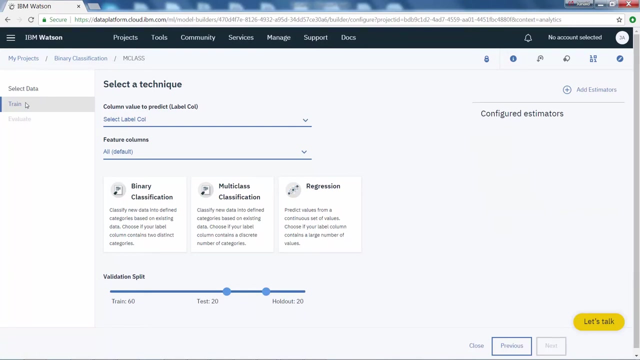 on the data and create your questions and have a very good idea what the data does. if you plan to prepare new data, keep in mind that it takes a long time actually to prepare a good data set. so here we are in the training section, and first thing is you got to select the column to be predicted. so we are interested in 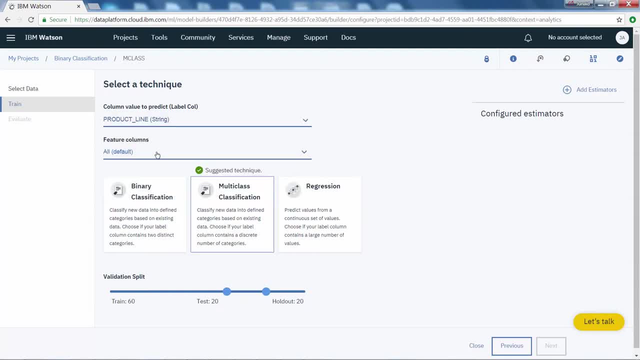 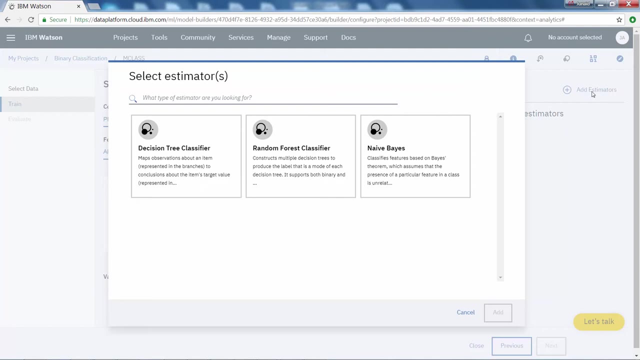 the product line and the feature columns are going to be all, so you're going to be in multi-class classification. now, as you can see, here you can actually add the estimators, which is basically the algorithm inside this category. so let's select all of them so you can train on all of them. 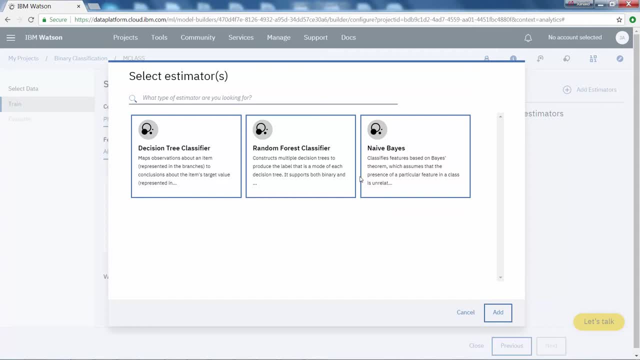 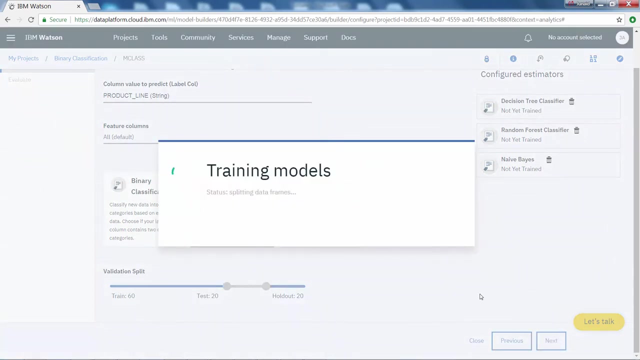 so that also will give us an understanding that, given the same data set, different algorithms will perform differently. so therefore a certain algorithm may perform better with a certain kind of data set. all right, let's say add here, and there you go and say next. so now it's going to start training the model. so this is going to take some time, as you have tree. 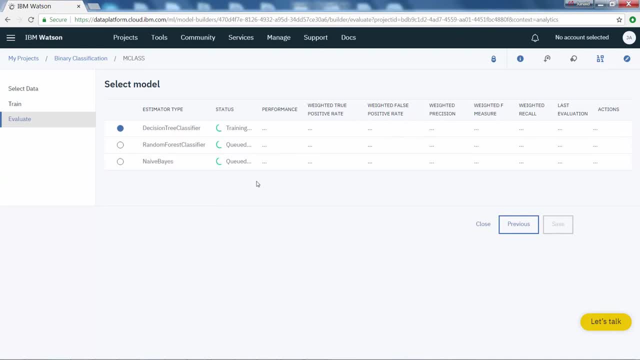 so this is going to go in a queue, so sit back and relax. all right, there you go. you have the training and evaluation done for you. as you can see that the different algorithms have performed differently, for example, the random forest classifier, let's select this one for now. has waited. position 0.9: weighted recalls. evaluate 20 points. gotten all the answers. so for each single classifier, just select this one for now and you can compare with the previous classifier. you can on a random plots classifier, let's say this one for now: it'sução lower than 400 shares. Holer TOP 30%. has waited, position 0.9, weighted, recalling, and then under the data�를 checkbox to check: is it out that data mean yes, area values? how can I, Sabrina, Elag difference down the bottom column? it depends on how. the error was a little bit different. so with this guy, which is not a smaller Polsce. 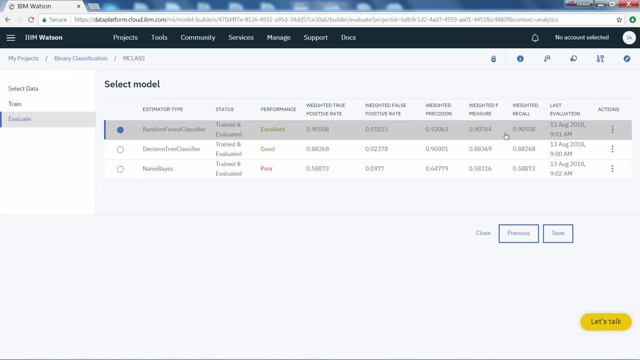 precision: 0.9, weighted recall: 0.9. and you're safe by looking at the weighted F measure. this is the harmonic average of weighted precision and weighted recall, so that's about 0.9. and then for decision tree classifier, this is 0.8. 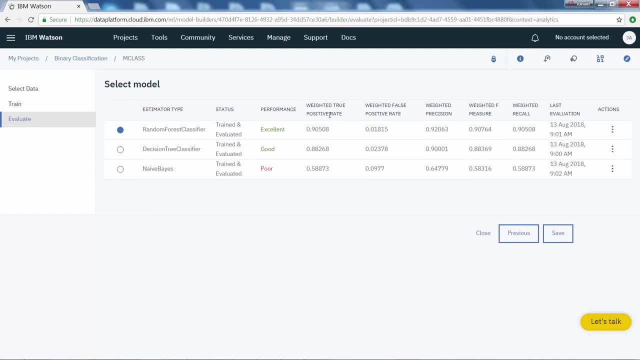 so please do take a look at the video for performance evaluation parameters, for a trained model, to understand these parameters better. now go ahead and select the best performance. so in this case, this is going to be random for a classifier and let's say save, all right. so now all we gotta do is deploy this.